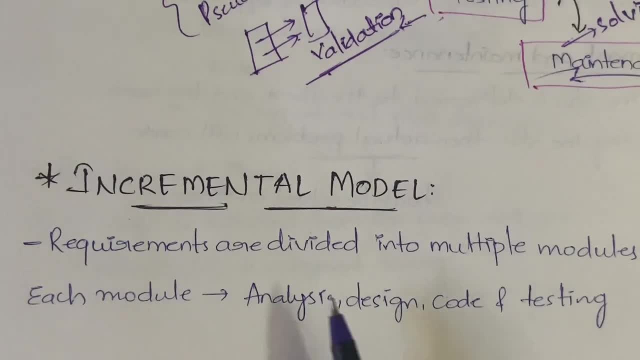 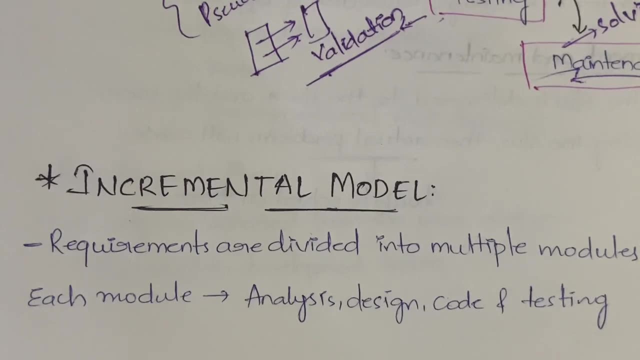 And each module, in each and every module, you will be doing the analysis, design, code and testing. okay, So actually, usually what we will do- analysis, design, coding, testing- we will be directly doing it, but here, instead of doing that, 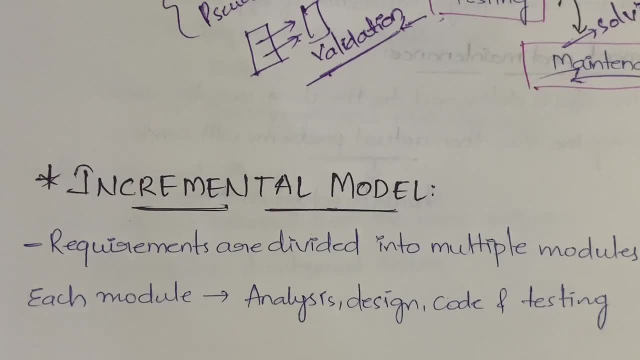 for example, we have taken electricity. so under electricity, what do we have? we have things like: what is the motto of electricity? electrician: when we are constructing the house, he have to provide the correct current supply and also everything he has to take care. so what electrician will do? 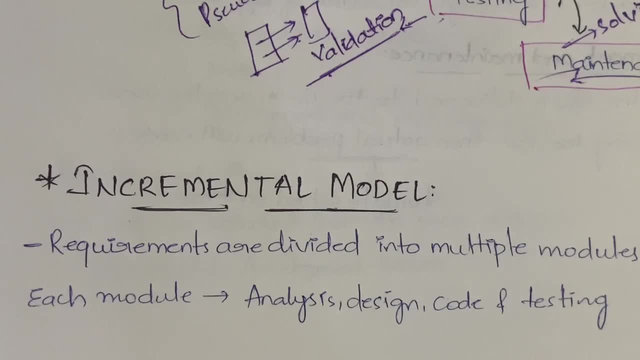 first he will ask how many sockets you want per room and which kind of sockets you want, which kind of switches. you want 20 amps, 16 amps, so like that. he will ask all the information. based on that he will do the analysis. so everybody is doing their specific, their separate, separate. 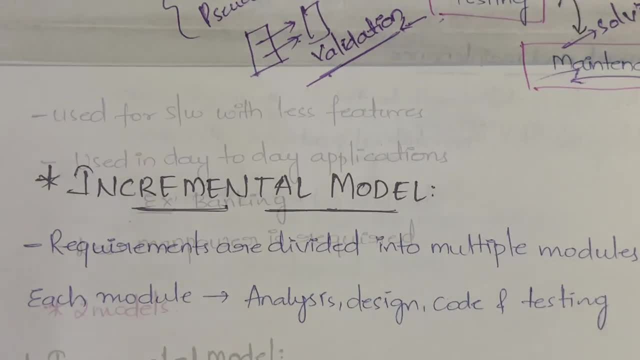 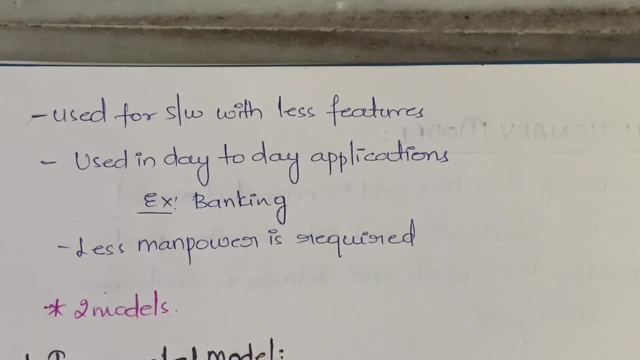 actions. okay, got it so with diagram, i'll show you. it is used in case of software which is having less features. it is used in our day-to-day applications, for example banking, and here we require less amount of manpower, since we are dividing the work. okay, and now here, actually. 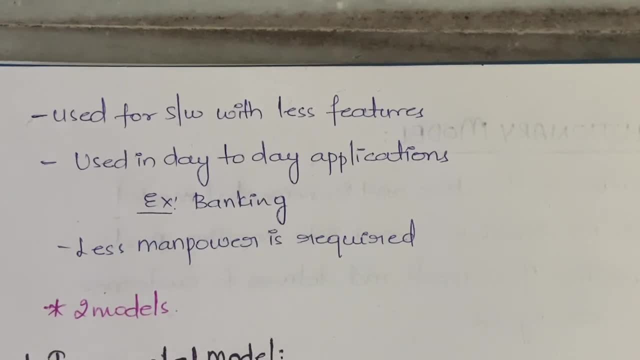 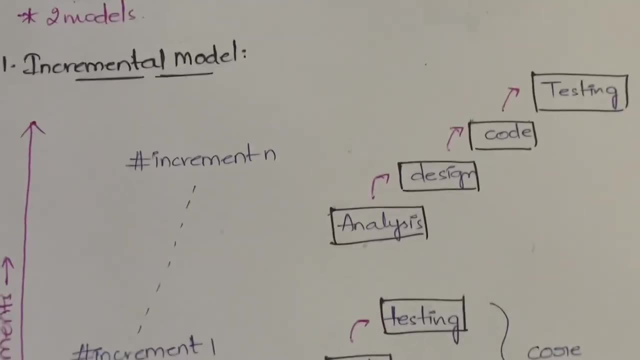 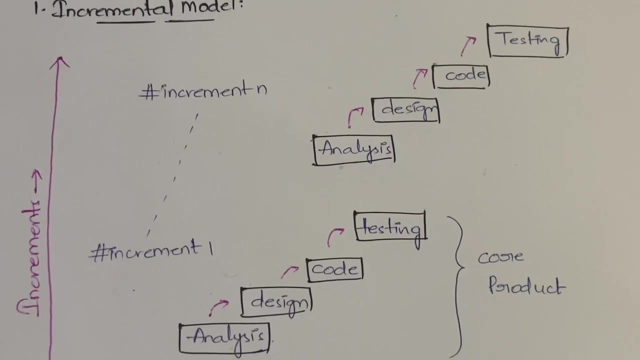 in incremental, we have two models, as i said in the process models video only: incremental and rad model. okay, incremental, first one, and the second one is the rad model. rad is nothing but the rapid application development. i'll tell you about both of them, don't worry. so here in incremental model, what you're doing is: 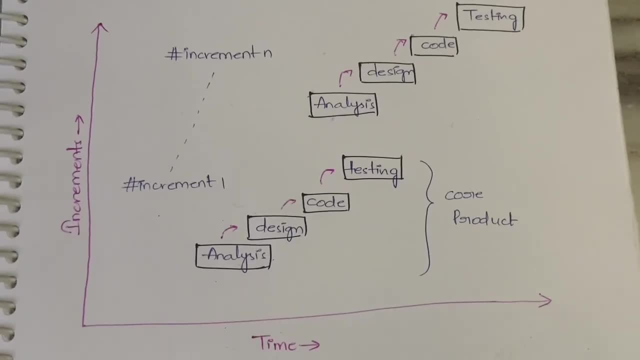 let me zoom in more. okay, fine, in the first one, in the incremental model, what you will do is: first you will have the core product. core product is nothing but the initial software. okay, this is the basic software, this is the increment one. you will have all the 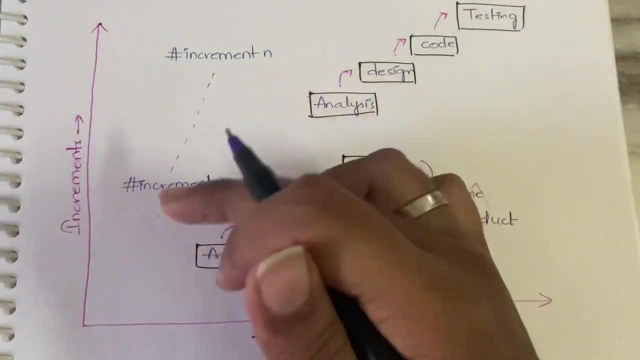 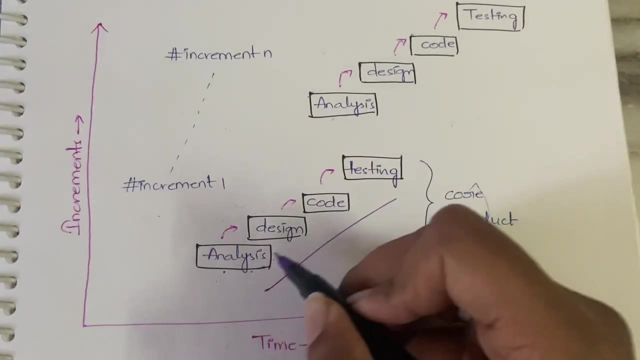 four steps in each and every increment, in the second increment, in the third increment, and so on up to n. in all the increments you will have the four steps. okay, so the first step is analysis, design, code testing. all these four will happen in the core product core. 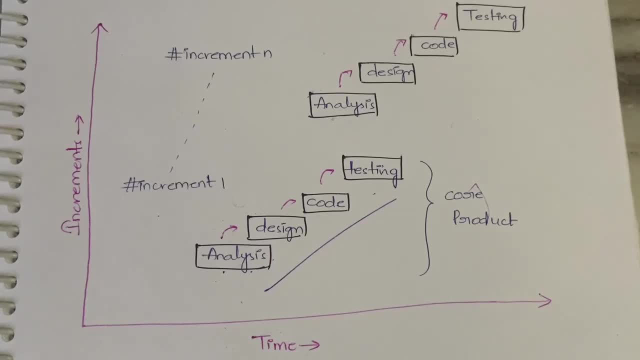 product is nothing but the basic software which you develop initially. and for this code products we keep on adding the requirements continuously according to our requirement and we will be enhancing it. got it? so the first increment is called as the core product. simply, you can remember in that way. 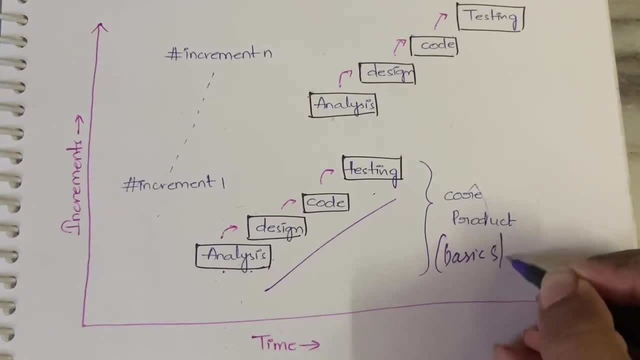 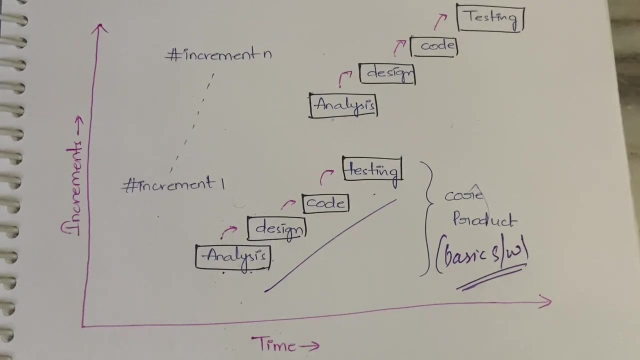 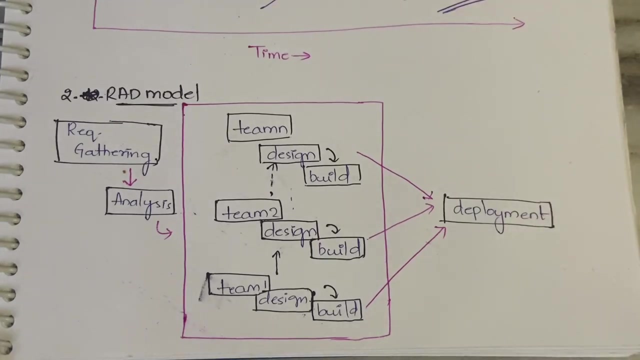 this is the basic software. okay, and for this software, in number of increments, we will be, you know, sequentially adding requirements and making it a complete product. that is what happens in incremental model, simple, okay, this is about incremental, very short. next let us move to the rad model, rapid application development. of course, this is also going to be very short, but why do you use? 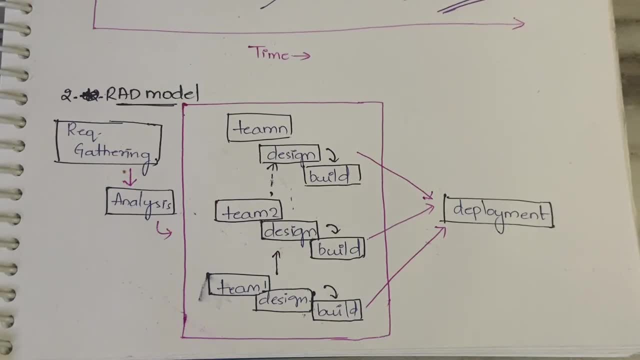 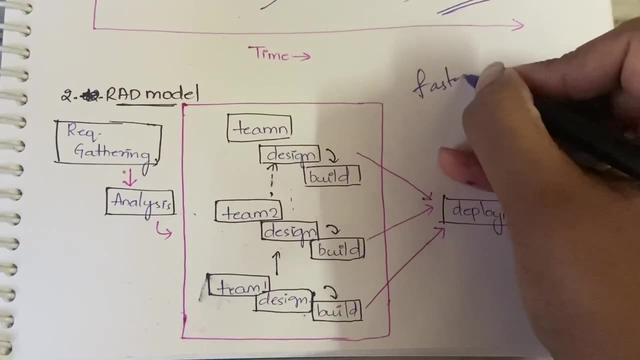 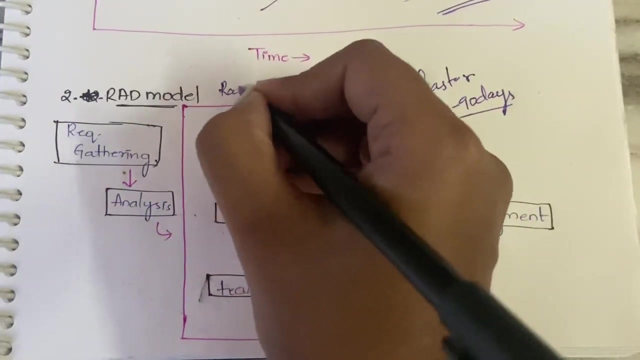 why do we have two different things here is, when you are having short period of time, when you want to complete it- complete sorry- when you want to complete the project faster- within 60 to 90 days, suppose then you will go for this rad model, rapid- rapid itself says right, fast application. 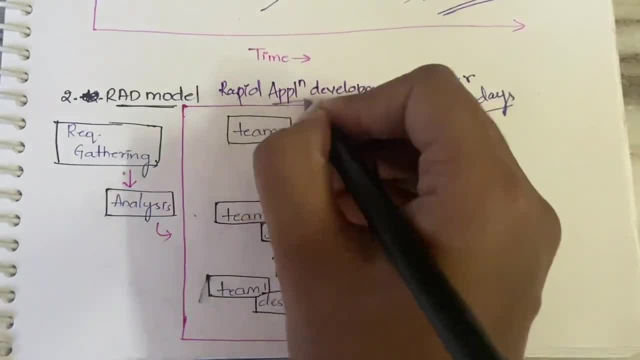 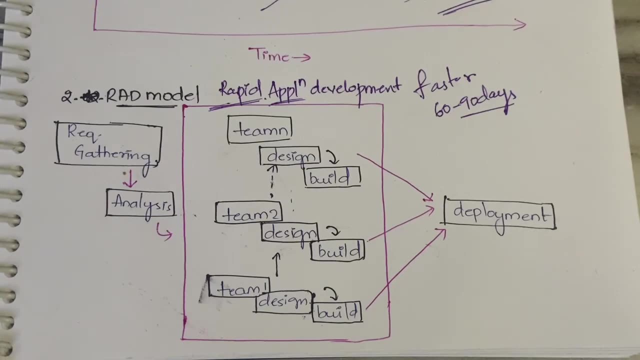 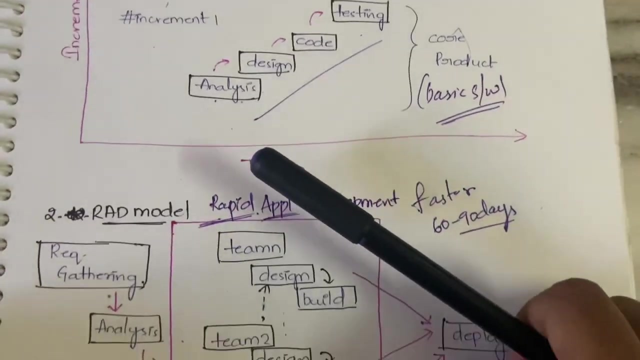 development. when you want to develop the application really very fastly, you go with this rad model. so here what is happening actually in incremental, in the top in here what we did: analysis, design, code, testing. all the four steps are done in each and every increment rate. it will take time because the first increment you have to 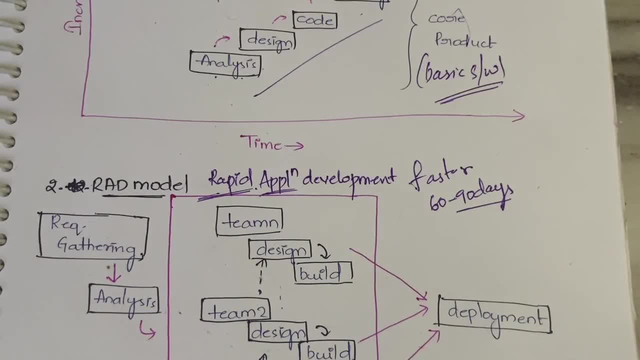 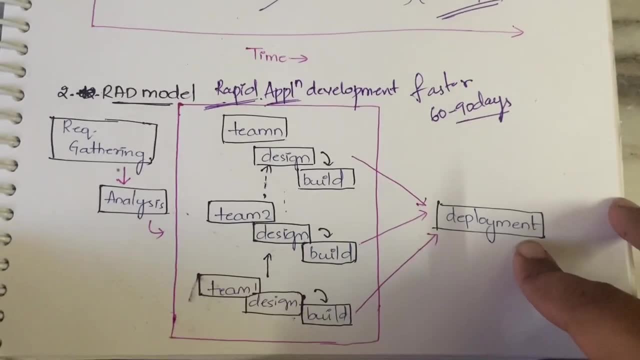 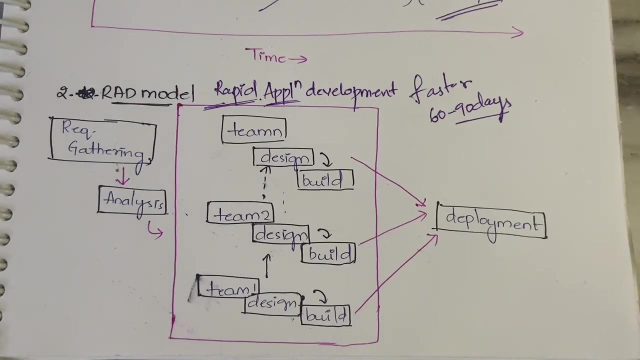 do the four steps, then you have to again see what are the requirements implemented and what are the additional requirements. then you have to do the second increment and all. but here what we are doing is requirement gathering. analysis is done only once, okay, and once you do the analysis after. 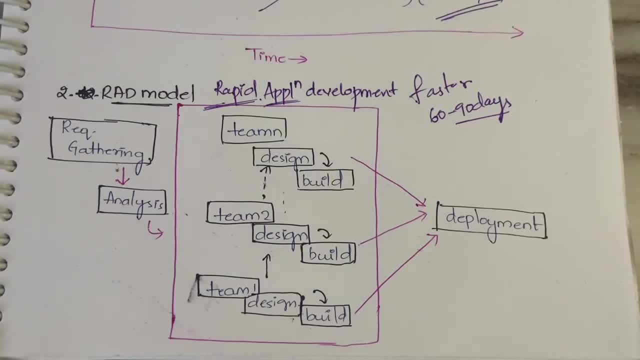 the doing the analysis phase. we are dividing the project into number of teams. okay, so again in our building, constructing the house, example one: instead of giving the complete responsibility to the electrician, what we are doing? we are only analyzing the tasks that are to be done by the. 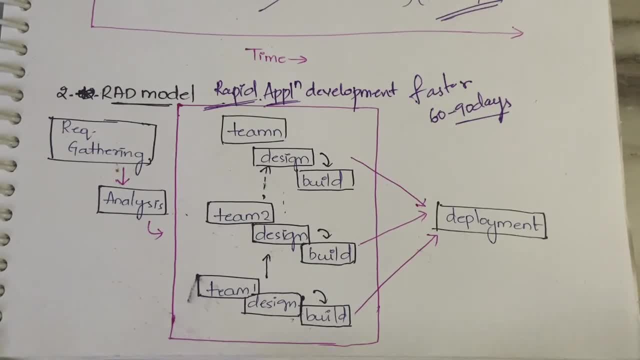 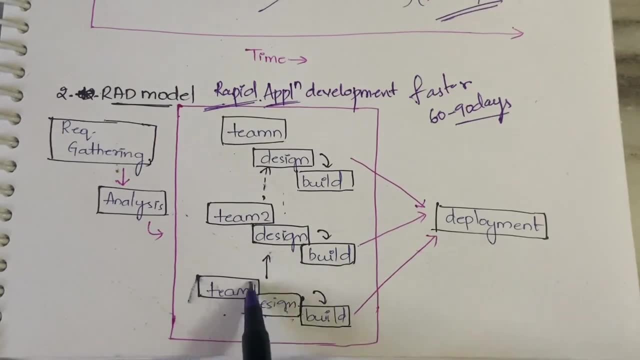 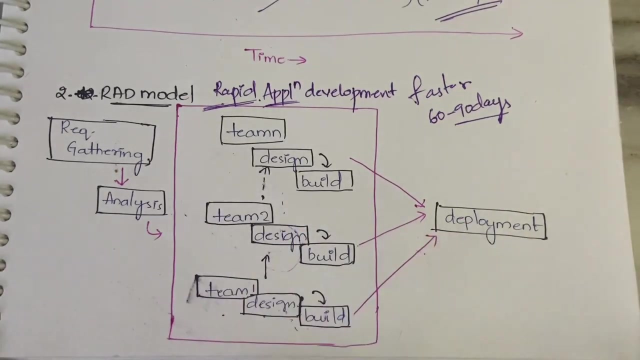 electrician and we are just giving him the task. okay, so we are assigning a team- design, build, and this team will design and build the software and give it to the next and also deploy, and this also will build and give it to the next. so that process will continue, okay, and all the process together. 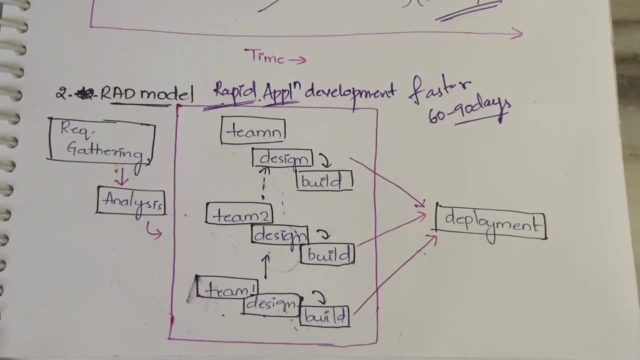 they will come and they will deploy the project. okay, so this is the difference between the incremental and rad. incremental will take some time. in case, if you want a project in less period of time, you can go with the rad model. but incremental or rad, whatever you want to choose.